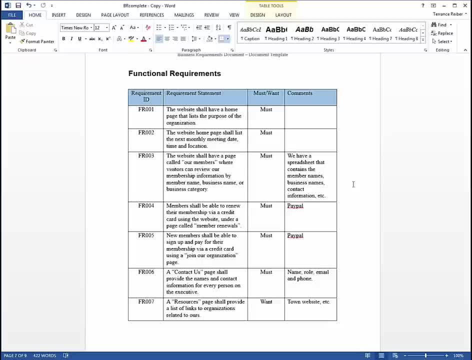 has a requirement ID. So then later on, if the business users come back and review these requirements and say I've got a problem with requirement so, and so you can say: well, which one? Oh, FR004.. Okay, everybody can turn their attention to FR004.. So it's always. 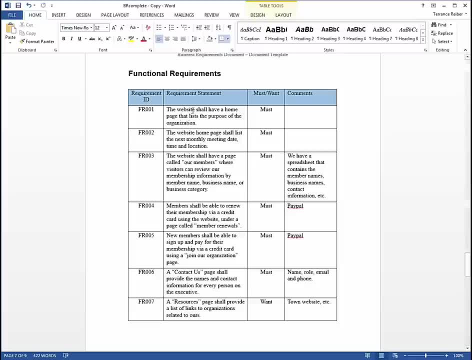 good to have a requirement ID associated with each requirement- Shall. it's a good practice. So, if you notice, all these requirements have a shall statement And then there's a must or a want. Must means if the solution can't do this requirement. 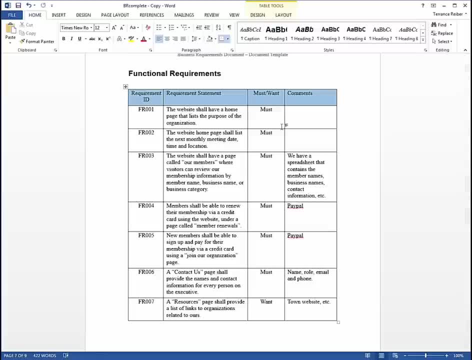 then that knocks that solution out. A want means it's kind of like a nice to have. So if you look at these requirements, they're saying they want a homepage that lists the purpose of the organization. Their homepage will list the date of their next monthly meeting. 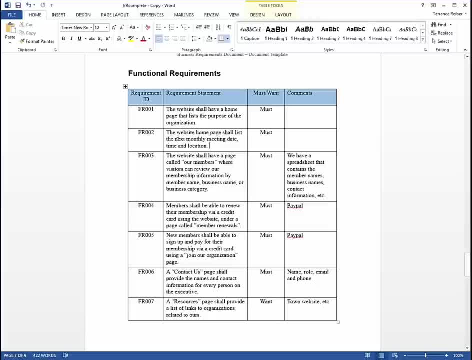 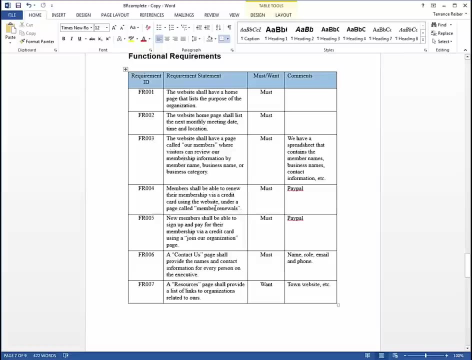 and their time and location of that meeting. This association has monthly meetings. It'll have a page that lists who the members are, sorted by various categories, And they go on and on and on And basically you just keep asking them: is there anything more you want? It's like a Christmas wish list And they 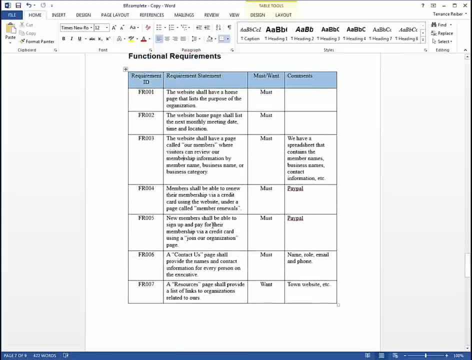 just keep coming up with requirements until they're done, And you can always circle back at the next meeting and just review them again and fine tune the wording of them or add more requirements. What makes a good requirement A good requirement should be measurable and verifiable. So when 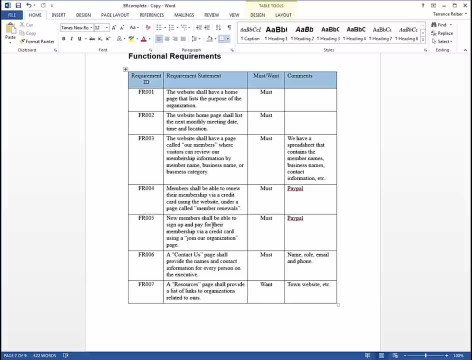 this website is developed by some company or person that makes a website. they can go back when it's delivered and say: okay, does the homepage have the purpose of the organization on it, Yes or no? No, Well, hey, you didn't get what you paid for. Yes, Great, We'll move. 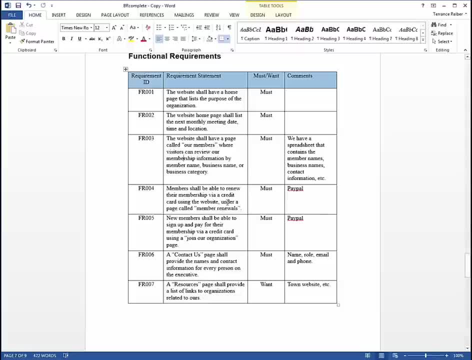 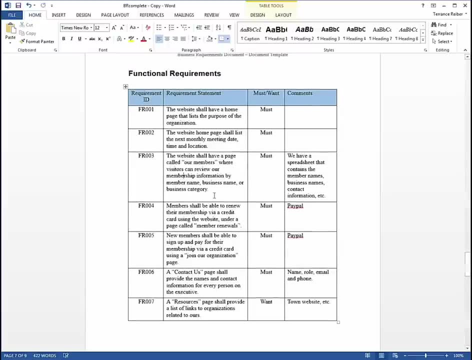 on. So requirements are there to make sure that the features of the site are there, to make sure that the system is delivered in the best way possible. These are called functional requirements. I'm going to have another video that talks about non-functional requirements And what's the difference between a functional requirement. 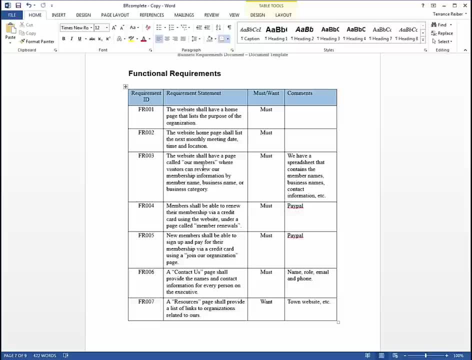 and a non-functional requirement. But for now, functional requirements are like features. They're things that you definitely want to experience when you use the system And it's great having a list of these because later on you can compare. let's say you're looking.